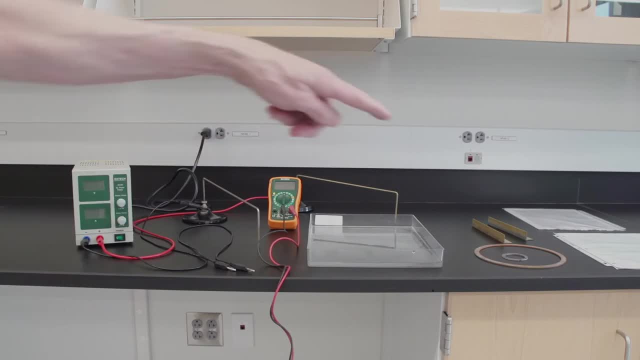 way to measure what the fields are, And we have various geometries of things. we can stick in there Some probes which we'll put in the water And some graph paper which we'll go underneath, so you can see where we're making measurements. 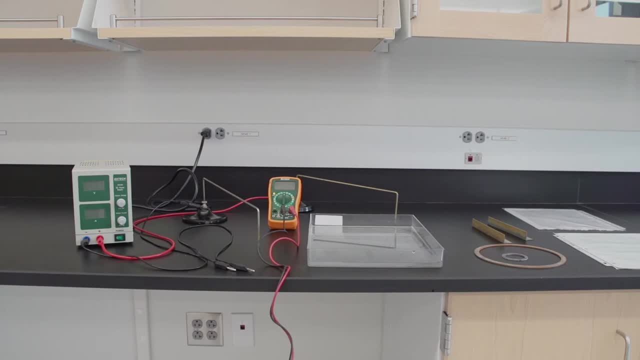 It's not very easy to see that from an angle like this with this camera, so I'm going to move all of this, put the water on the floor and we'll look down on it so you can see it better, And then we'll make some measurements on it with different geometries. 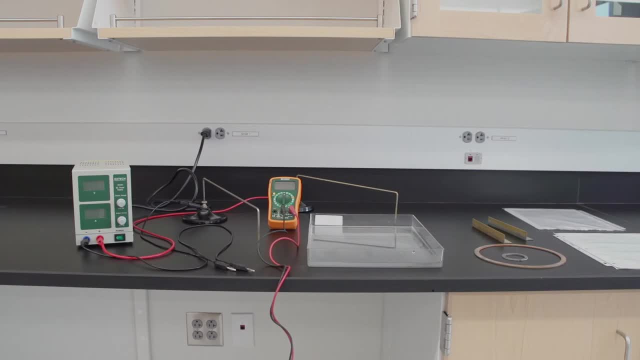 Before I do that, let me just point out the voltmeter. It's a standard laboratory voltmeter, so it's one that you may be familiar with already. You can go to Home Depot and get one of these things if you want one at home. They're not very expensive anymore. they used. 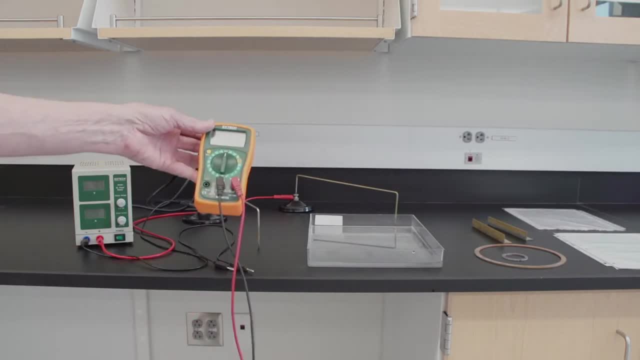 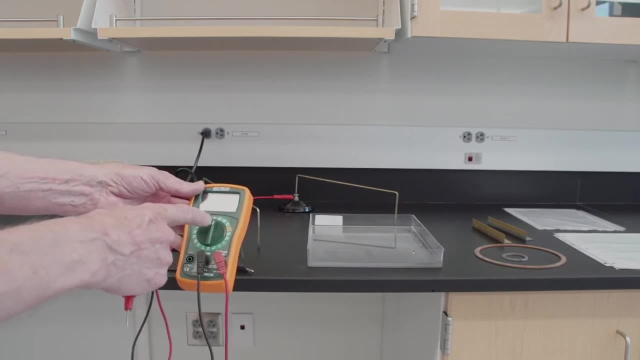 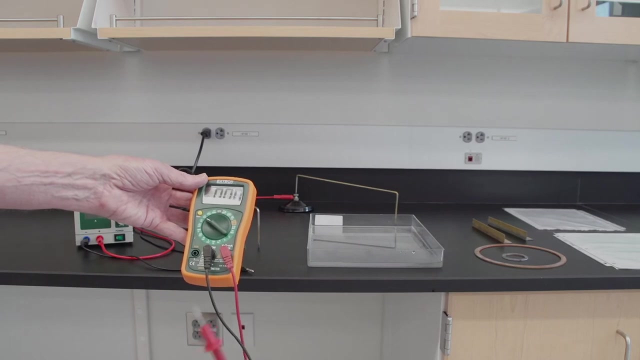 to be. So we have a couple of wires here. One's connected to common, The other to the volt connection for the input on this meter, And then a dial which lets us select what it's going to measure. If I put it over here at 20 volts, 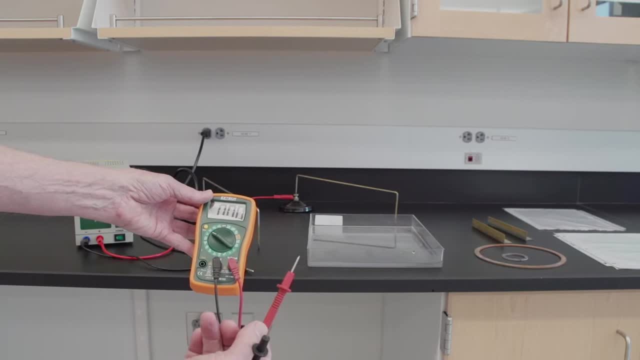 between the two ends of these probes is what is seen on this meter up here, measured in volts. A lot of physics inside this device, good basic electronics, and so you just have to trust that that's actually what we are talking about here. It will also measure current and resistance and a lot of 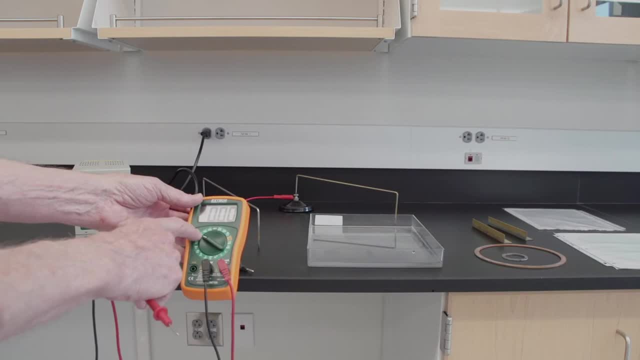 other things. We're going to use it in this simple mode, set to 20 volts, and these two leads- common usually means ground. in this case it'll be zero, and then, with respect to that, the red lead will be plus. In order to use this with, 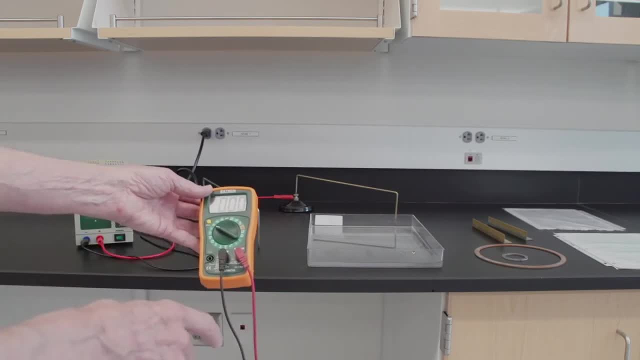 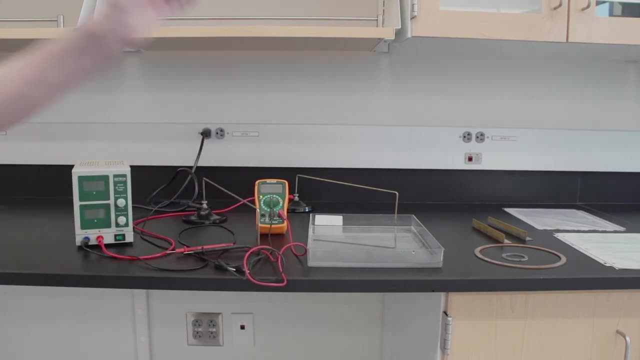 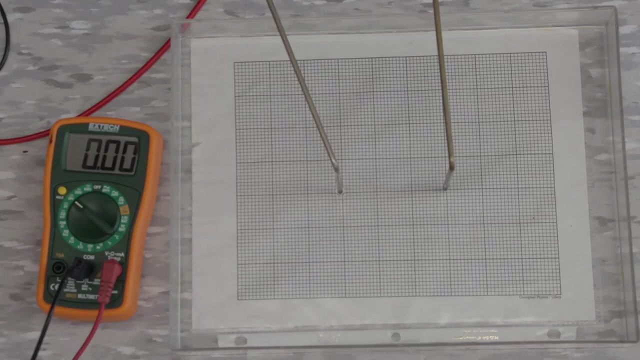 the water. I'm going to connect this lead over to our power supply and I'll explain that in the next part. So now we've set up this pan of water, We're going to use it to measure current and resistance With electrodes in it. you can see, I can touch the water and it demonstrates it's there. 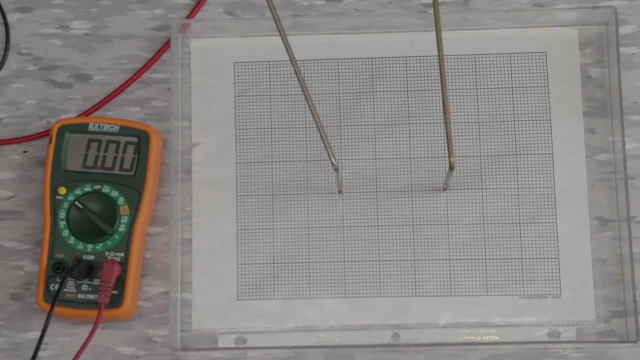 conducting. Underneath the pan there's a grid of graph paper you can use to measure the position of a probe. I can move around. this probe is connected to the voltmeter and these two points are connected to the power supply. this one 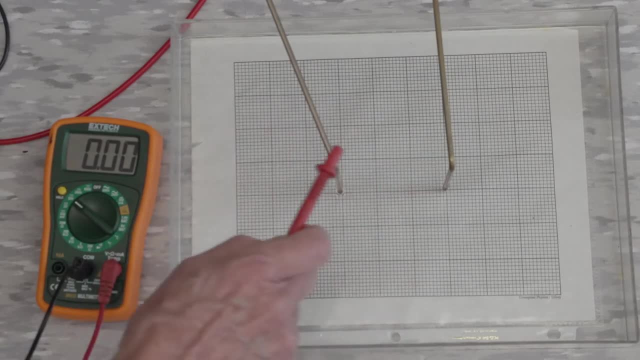 to 0 and that one to plus 10 volts. If I touch this you'll see 0, but if I touch that you'll see 10 volts. If I move the probe around, you'll see different voltages here in the conducting water. So take a look at that graph paper and 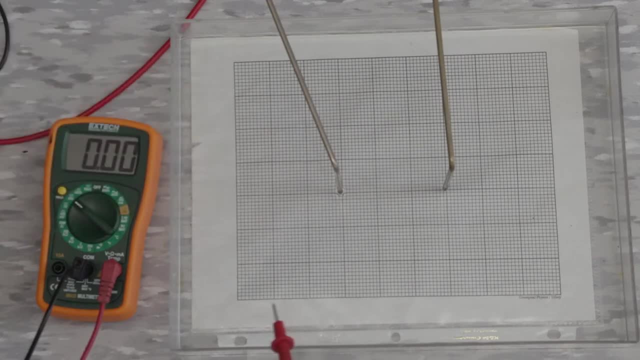 decide on the coordinate grid that you want to use. I'd suggest you use X in this direction and Y in that direction, And I'll touch this probe at various places and you can make a note of what the voltage is in these different spots. 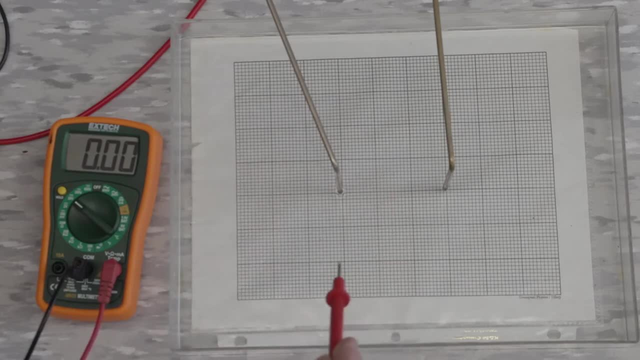 I'm just going to sample as best I can, all around this area and we'll see what we get. So let me start down here and I'll just go across. We'll go back again here on the left and go across, And here and there We know that one's zero, Here and here. 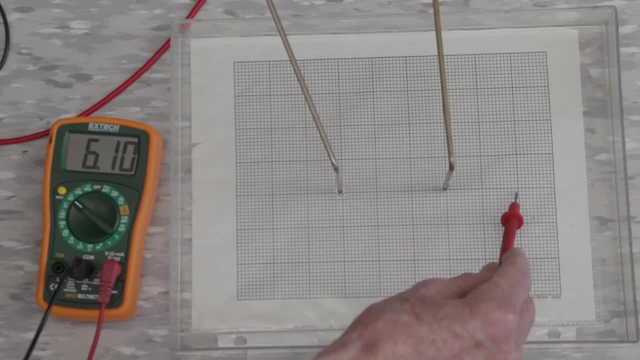 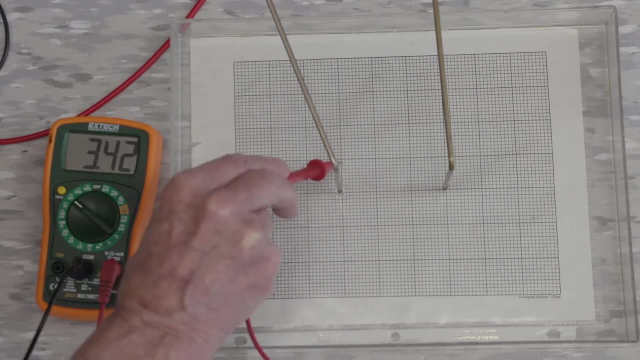 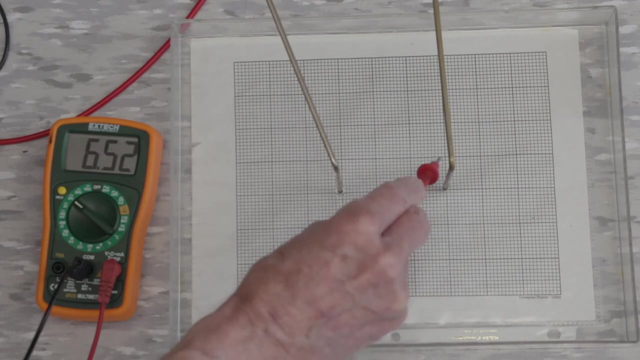 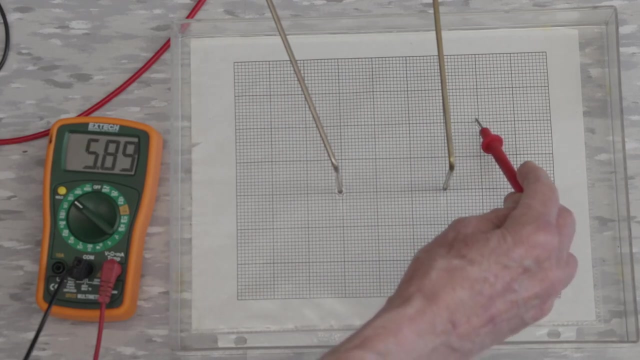 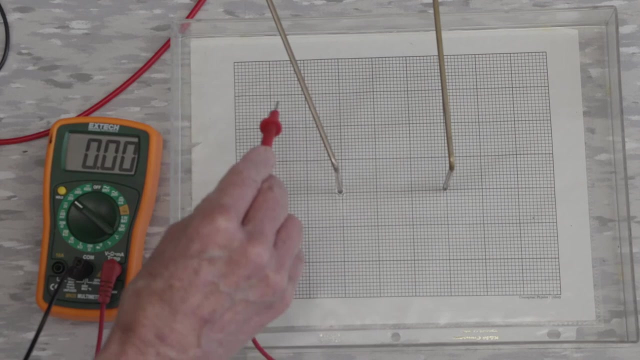 And there And there, We'll go up here, Going up here. So we went down two and up two and back and forth. this way Let me see what happens if we go down the middle here. So I'm just going to try to find the center. 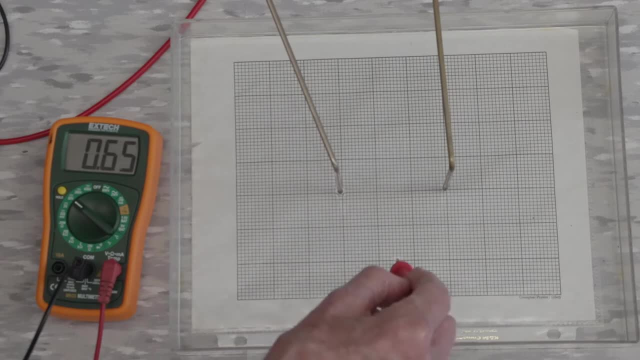 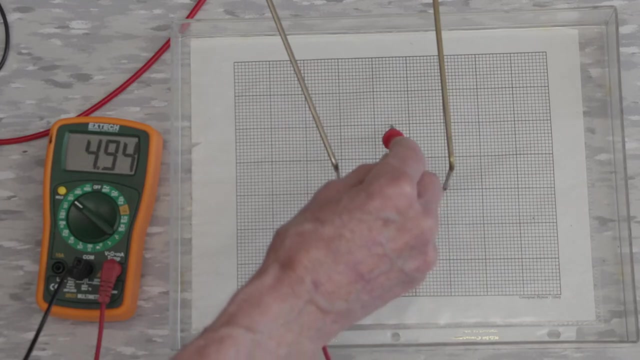 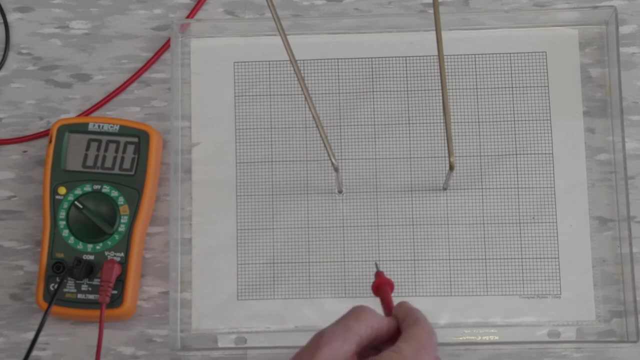 position. It's nearly the same all the way down there. That's an equipotential. The potential is constant along that line. What if I go over instead of being exactly in the center? go over, and so I'm a half a space over from zero here. So we'll start down. 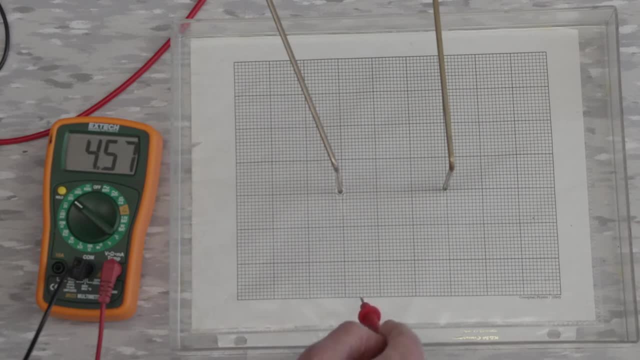 here at the bottom and just go up. You see, those are not constant, So the equipotential runs straight up and down through the middle, but over here it doesn't run straight up and down, In fact, if I take that point right. 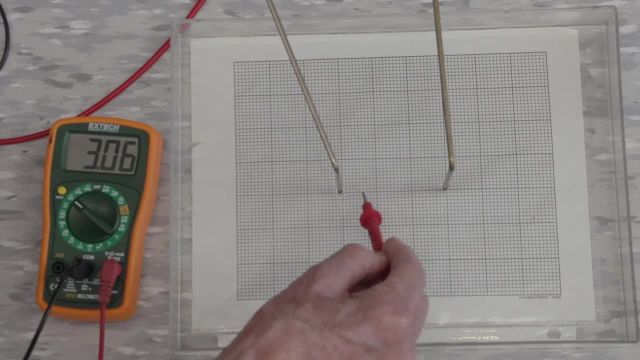 there I've got 3.2 volts. Let's see if I can find another 3.2.. Searching for it here. There's one right there. I'll go over here and see if I can find one Like that. Here's one. 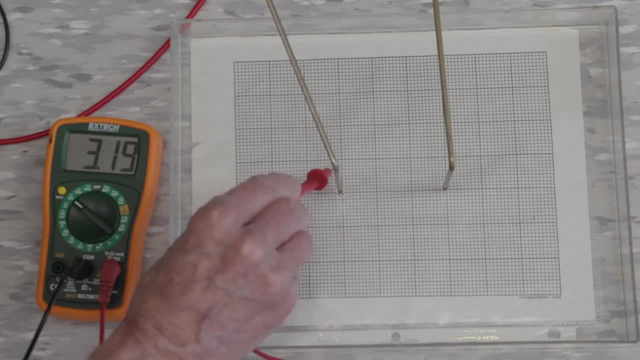 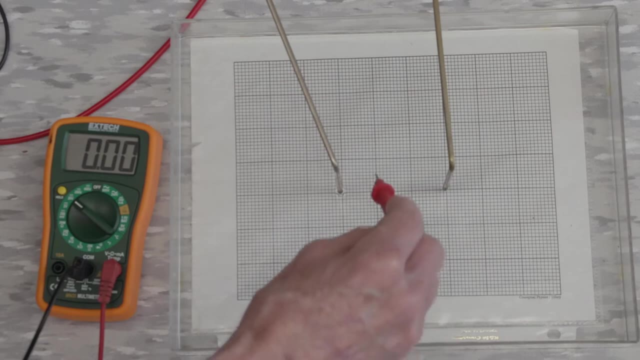 Up here, Like that, Maybe around over here somewhere, In there someplace. So the equipotential near this point is a circle, or nearly so. around that point It's not quite a circle. If you plot those out you'll see it's not exactly the same. 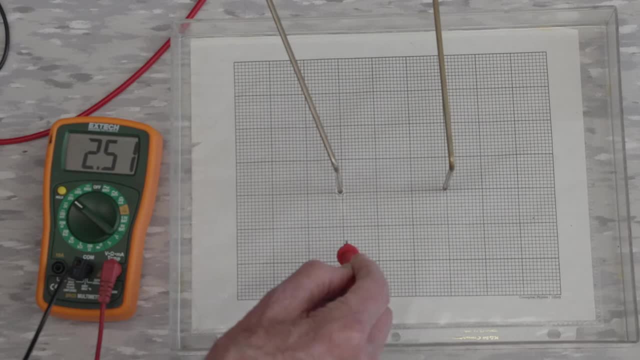 Let's come down a little bit farther. Maybe we'll look at this point right there and see what we have. That's 4.0.. So let's see where 4.0 goes. If we go down here, it's too much. 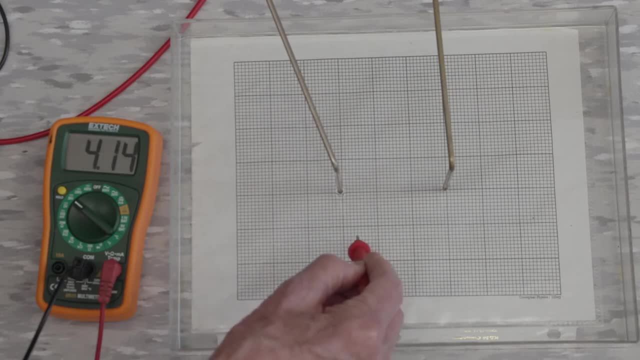 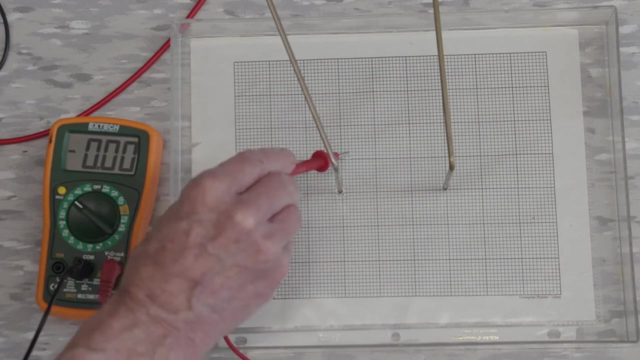 So I'm looking for 4.. There's one up in here, Maybe about like that, Right in there, somewhere, Right here, Over here, maybe Up here, How about down here? So that 4.0 is not a circle, It's some kind of a curve which comes around that way. 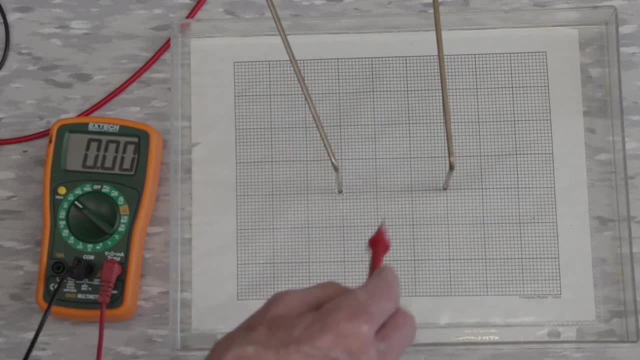 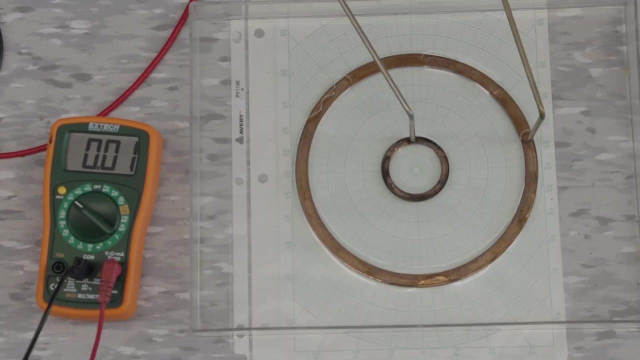 So we've measured the potential on a grid and now you can get a sense of how the lines might curve. See if you can take those data and figure out what the equipotential lines look like around these two points. Now we've changed the geometry. 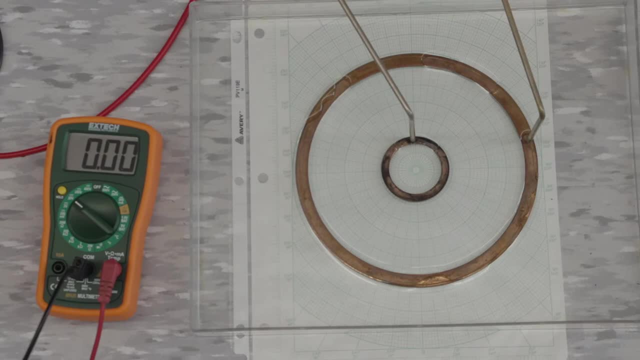 We've put two circular rings- These are actually copper rings- in the water- And to make it simpler to measure, I've put a piece of polar graph paper under the track. So we're measuring with respect to a polar coordinate system. The center of the coordinate system is now in the center of the inner ring. 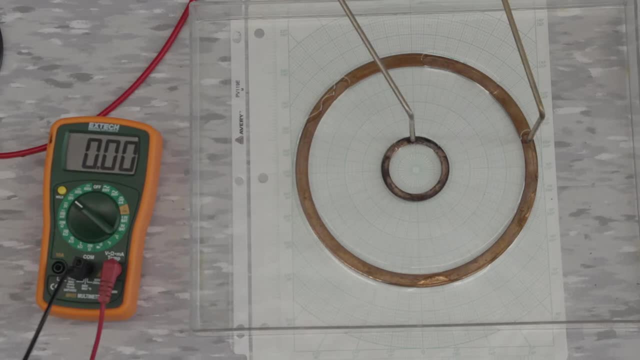 The inner ring is 2 inches in diameter on the outside. The outer ring is 6 inches in diameter on the inside. So if we look at the spacing between the inside and the outside, we have 1 inch from here to here. 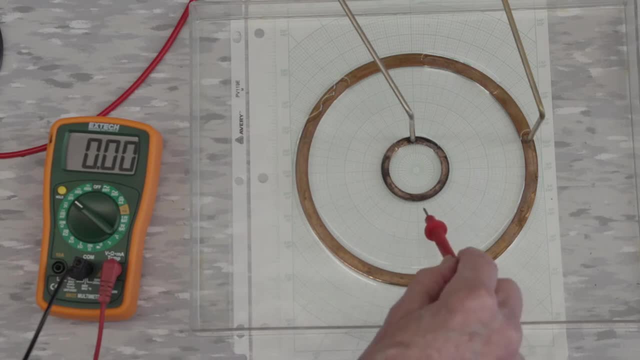 We have 3 inches from here to here, So from the inner edge there to that edge is 2 inches, And these grid marks are in half inch spacings. You can measure even to a tenth of a division using those grids, If I put the probe in. 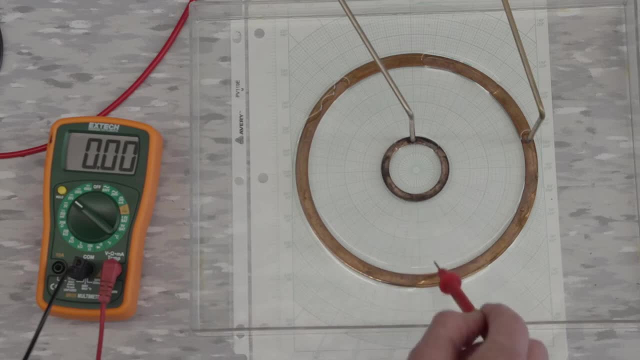 you'll see, it measures a voltage, because that's at 0 volts And this is at 10 volts. Let's see if we can find some equipotentials. Let me just put it right there: 7 volts, 6.7. 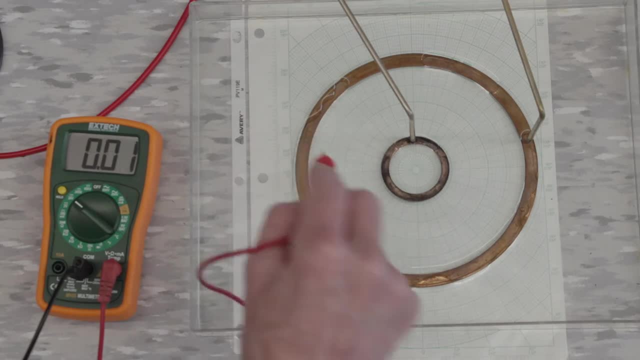 7, 6.8, 6.6. It should be exactly the same, but it won't be quite: 6.7, 6.9, 7. So let's just trace out where the 7 volt line is. So I'll start here. 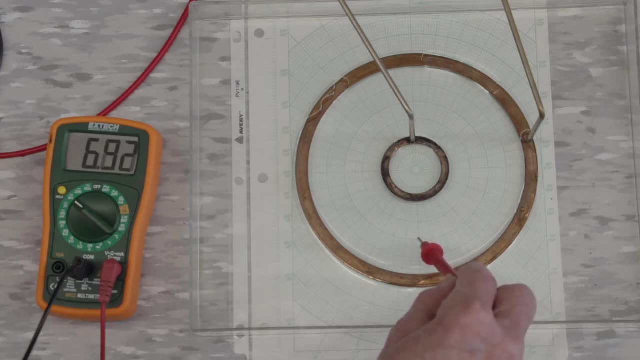 Let's see if I can find 7 volts, Make a note of where that is on the coordinate grid And then go over here. 7 over here somewhere. Find it right there. Try it out here. It's right there Up here. 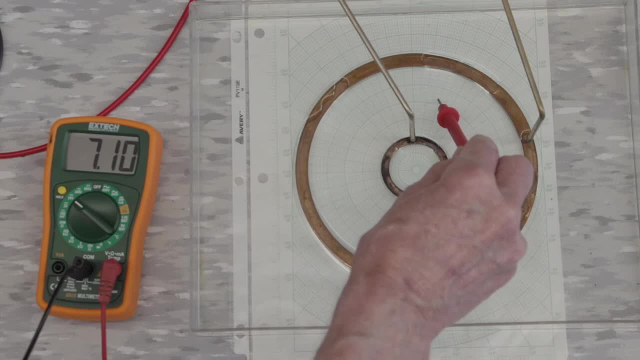 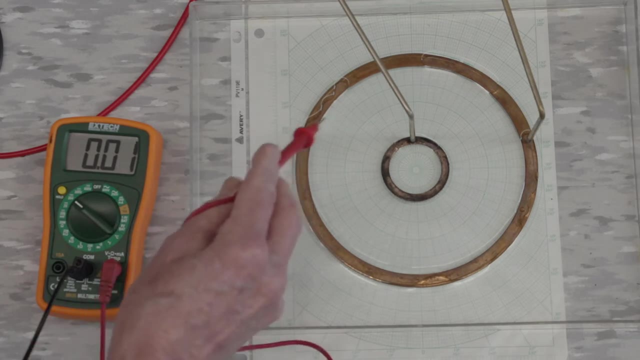 It's right there Up here. It's right there, So it's bulging out in that upper direction just a little bit. Probably a slight difference in contact around Up here 7.. 7. Down here again somewhere. 7, right in there someplace. 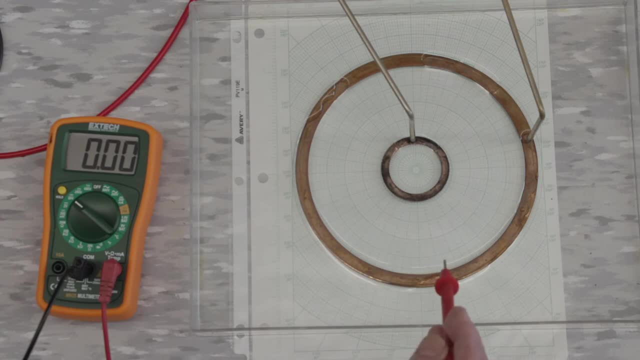 So to measure the position, you can go back and look at this video as often as you want. You use the radius outward, The radial coordinate of a polar coordinate system, So 0 here And, as you come out, that would be 1,, 2,, 3.. 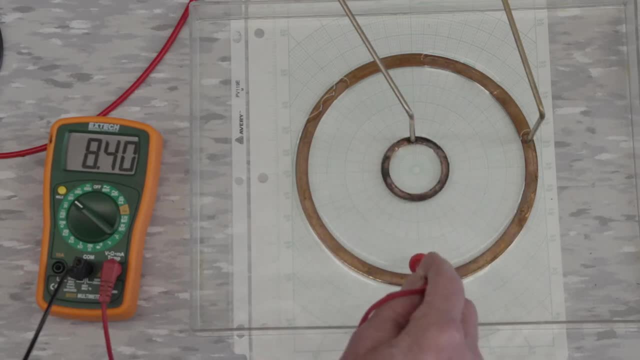 And then around in this direction. it's in degrees, So this would be 0 degrees. There's actually a scale which you might be able to read: It's 0 right there, 90 degrees here, 180 degrees up, 270 degrees over here. 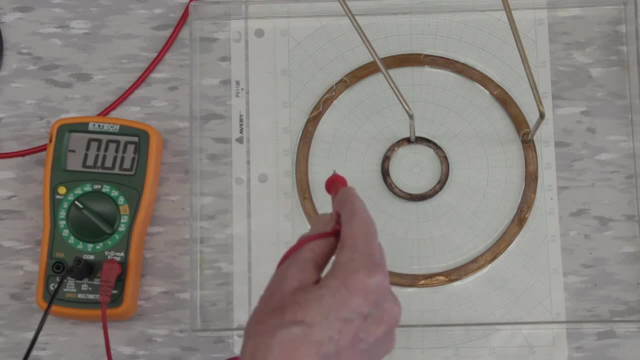 And these marks, the major ones, are in 10 degree increments. So that's 270.. 280.. 290.. This is 0.. 10. 20. 30. And so on. So let me just come down along a line here at constant 0 degrees. 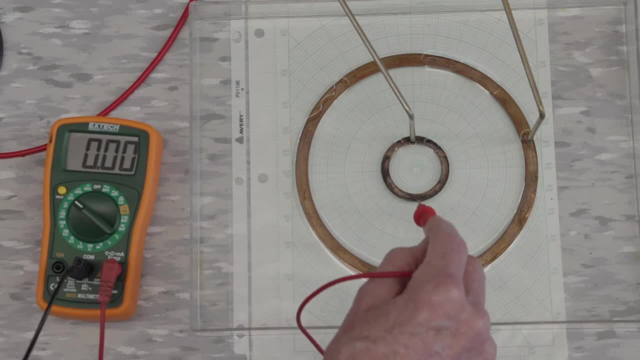 We know that on that surface I don't want to touch it because it might move it, But it will be 0 there. Let me just come out and I'll put it here. That's on the 1.5 mark There. 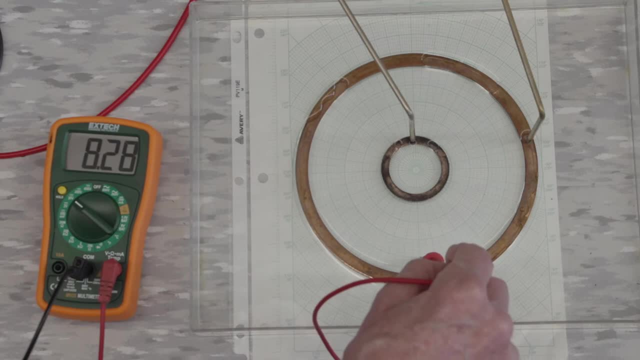 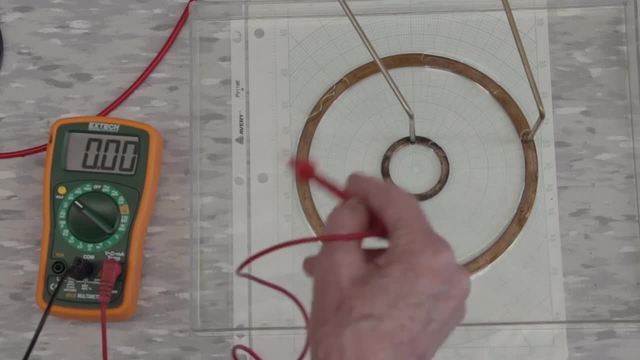 Let's try it over at another angle. It should be the same because it's symmetric around. in this direction It shouldn't be any different. But if there's a little difference in contact that changes the voltage on the outer circle in various places, it might be different. 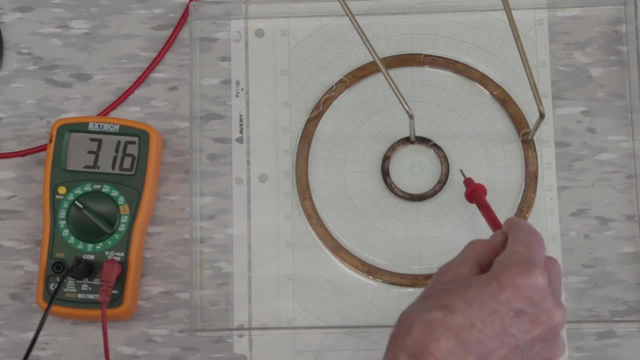 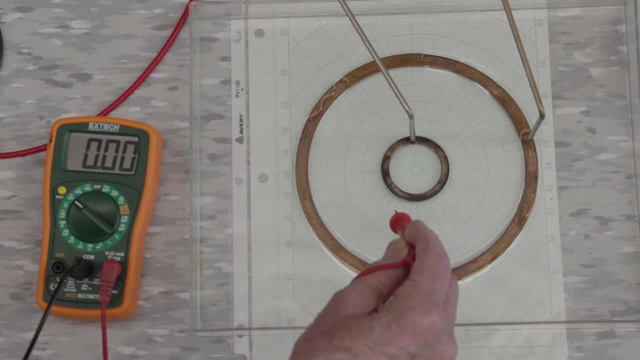 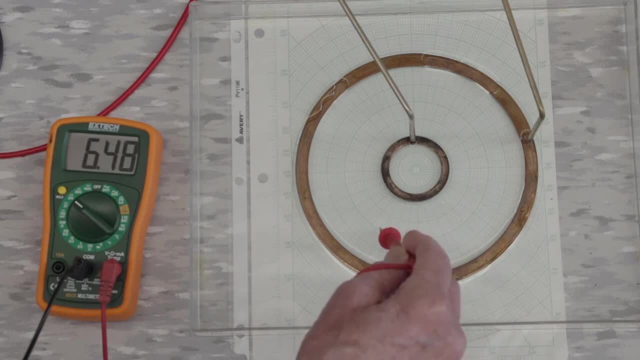 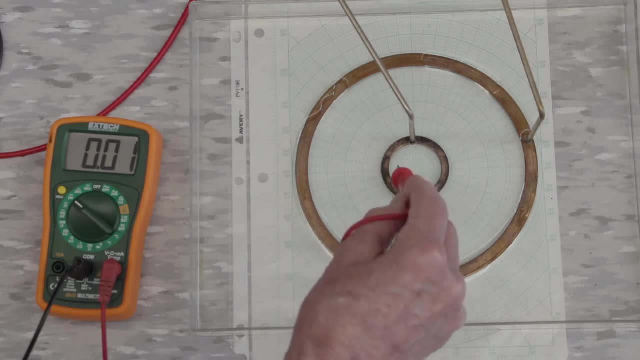 There. So again, that's 0.51,. this is 1.5 here. so a radial distance out, we have one there and then this will be two and that will be three. so we start at 1.1, two, three, four. 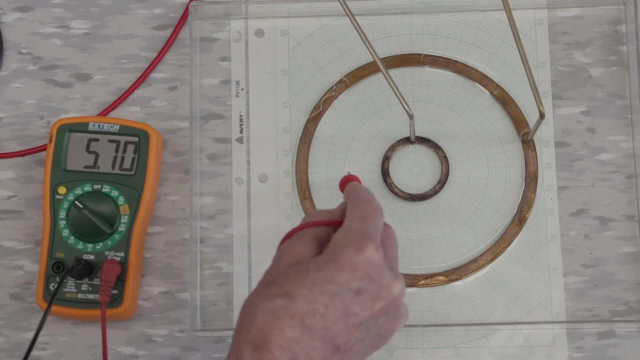 seven, eight, nine, and that'll be two, And then two point one, two, three, four, five, six, seven, eight. as far as I can go, Repeat it again, I'm just going to come down here in. 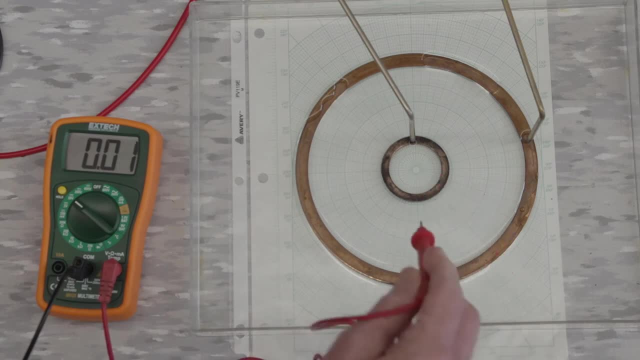 the middle, where I can reach it easily. At the end of the probe I'll put on a grid mark. So that's zero. this is one, and I'll go to one point. one, two, three, four, five, six, seven, eight. 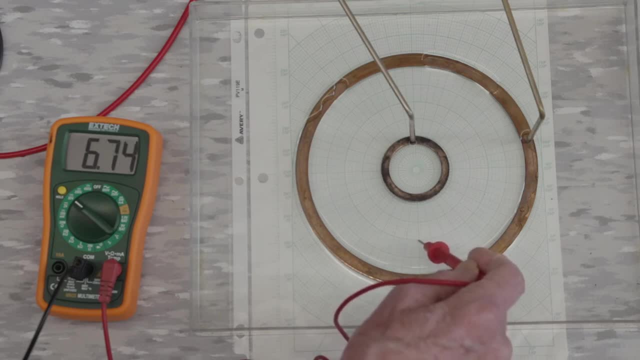 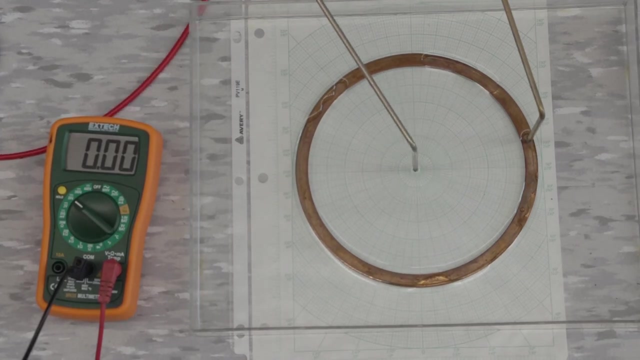 nine, and that's two, Two point one, two, three, four, two point five, two point six, two point seven and two point eight. Zero and ten. So now we've changed the geometry again. Instead of having an inner ring, we've just got an inner point. Again, this point is at zero. 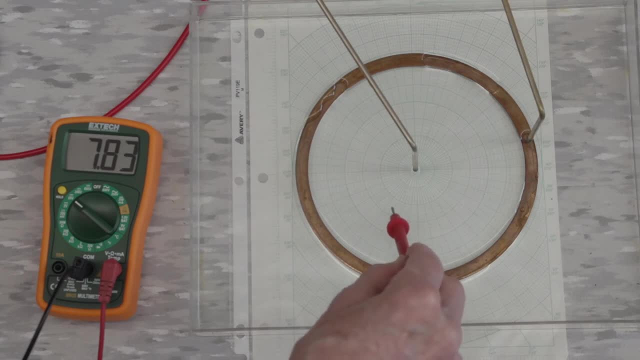 and that's at ten, And if I put this in here you can see how the voltage varies with position. So let's start out here at the middle. So it's zero if I touch that, but if I come away a little bit it's not. In fact, if I come out here to half. 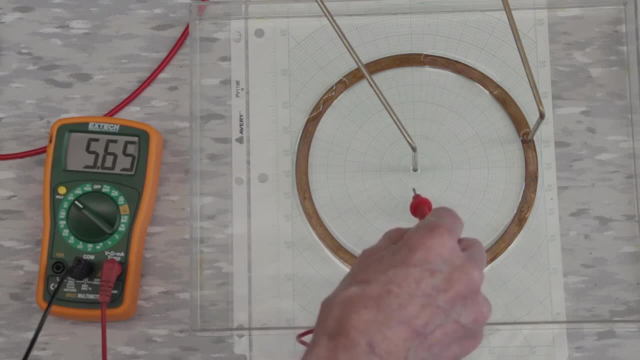 it's five, point, six, seven. So I'll start at this point, because I can't locate it very precisely in here, and let's just see how it varies. The probe is at point five, And then six, seven, 1.1,, 2,, 3,, 4,, 5,, 6,, 7,, 8,, 9, and we're at 2.. 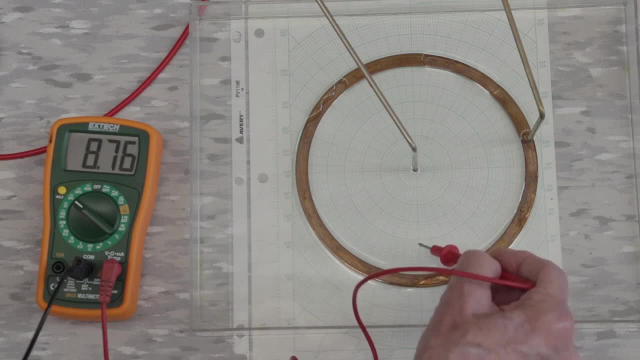 And then 2.1,, 2,, 3,, 4,, 5,, 6,, 7, and 8. It'll be 10 out here on the outer ring Inside here. there's a little meniscus around the end of that. 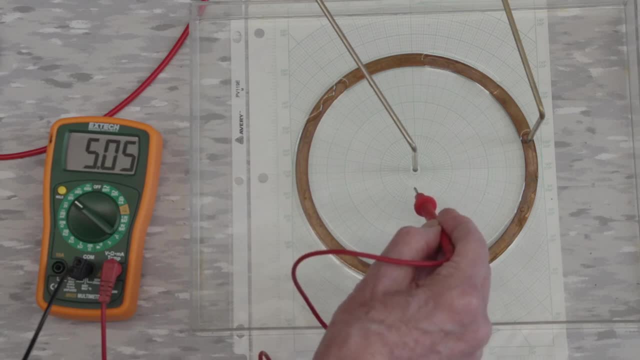 which probably affects that voltage a little bit, And I just can't go in, but let me try. So that's on the 0.5 mark, And then that's 0.4.. And then that's 0.3.. 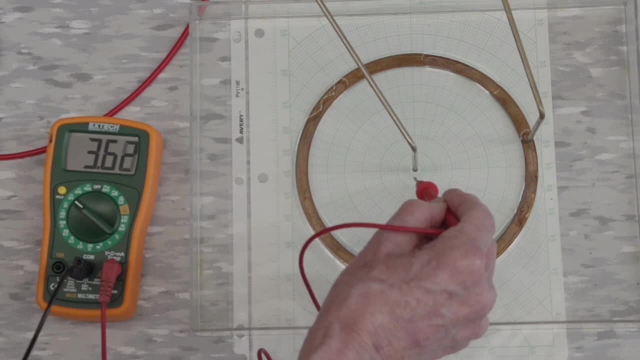 And it looks like that would be 0.2,, but I'm not sure. So you can experiment a little bit with whether that makes any sense. It's symmetric around this. because of the outer ring being symmetric around that point, It doesn't make any difference which radius I work on. 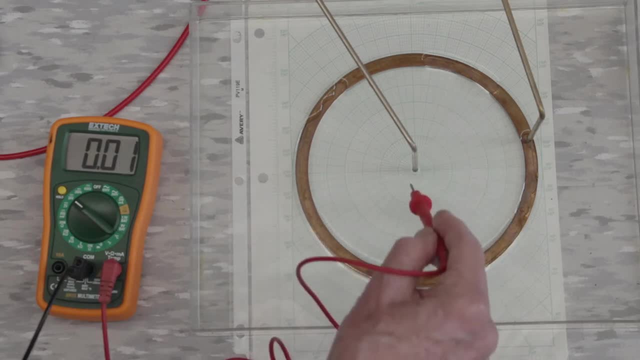 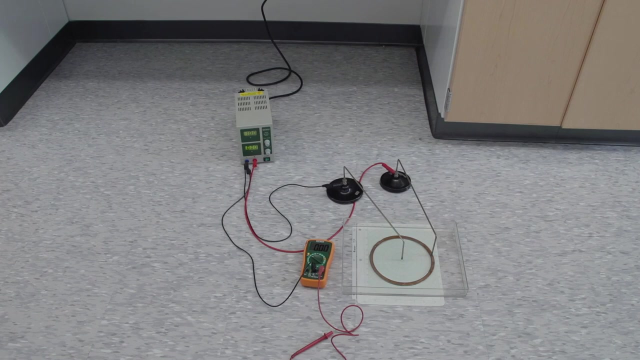 whether it's over here or there or there, It's going to be the same, so it's easy for me to reach right there. So, to summarize what we've done here, we have a power supply- and you can see it in this wider view now: 10 volts. 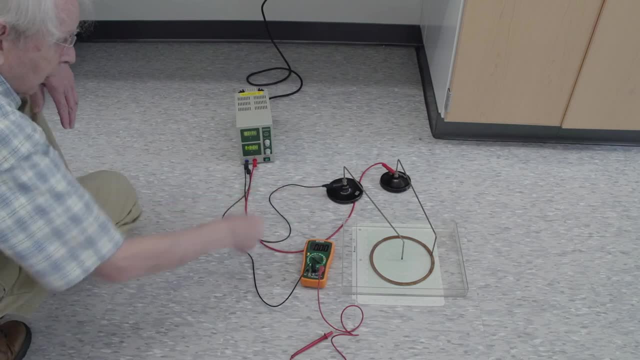 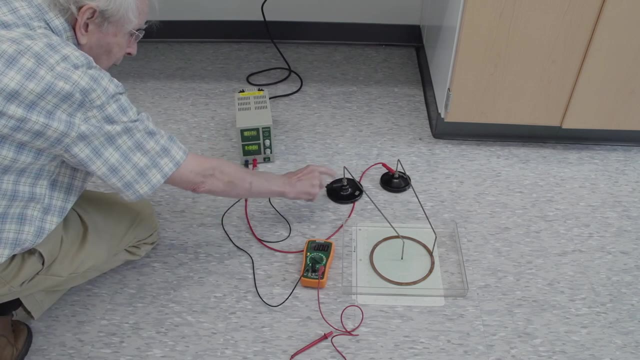 And the power supply puts 10 volts on this wire which goes over to this probe right there, And then in the middle we have another probe, which is this one which is at 0. So we have 10 volts ground and we have a voltmeter. 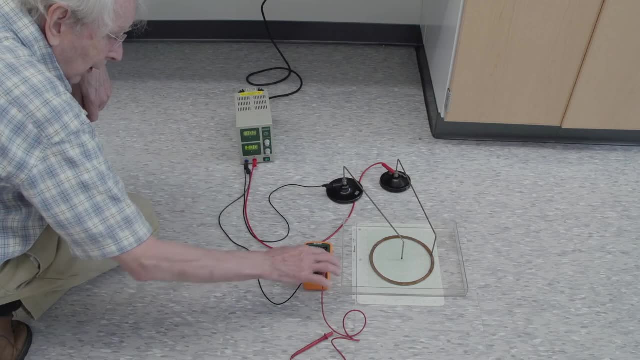 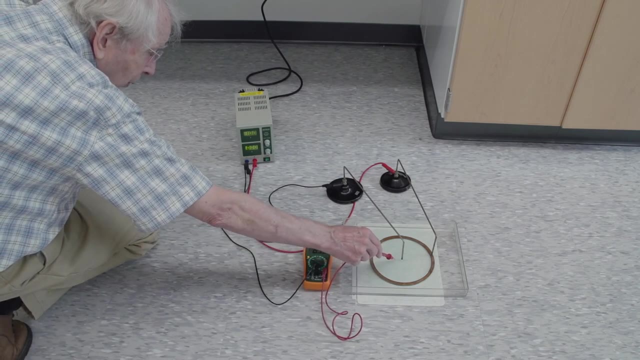 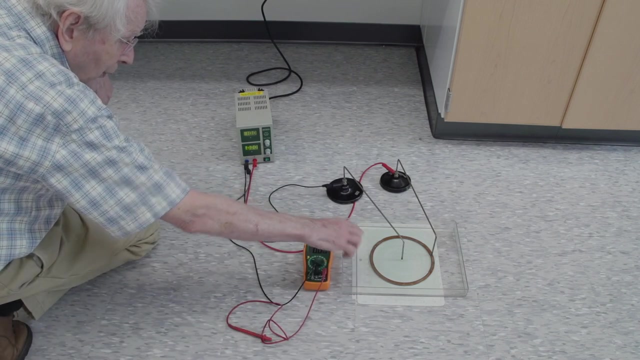 The voltmeter is connected to ground And the other lead of the voltmeter is a probe that I've been able to put into the water in various places to see how the voltage varies with position. This little pan has water in it and we've tried various geometries.